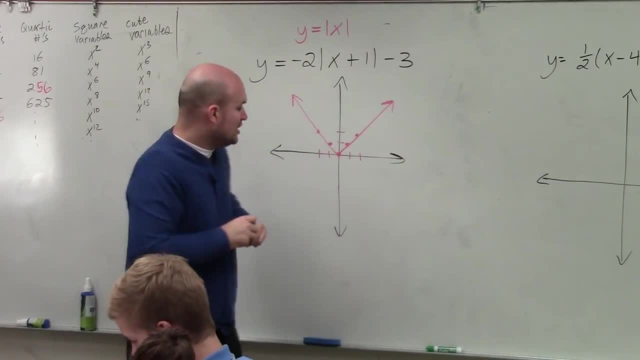 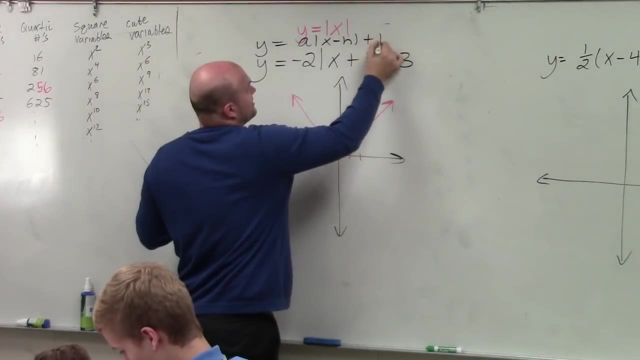 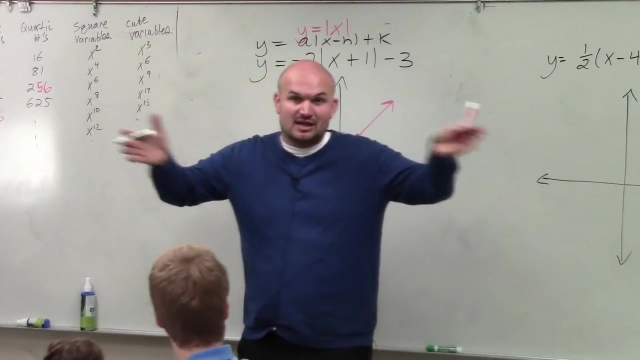 we need to do is look at what is the transformations. So to understand the transformations, we need to understand or remember: Y equals A times absolute value of X minus H plus K. Remember A either compressed or stretched the graph right, H shifted the graph left or right. 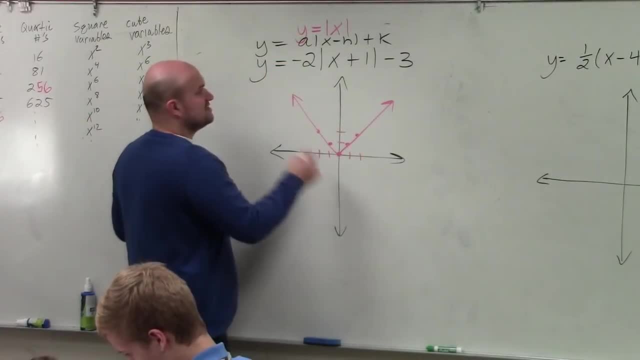 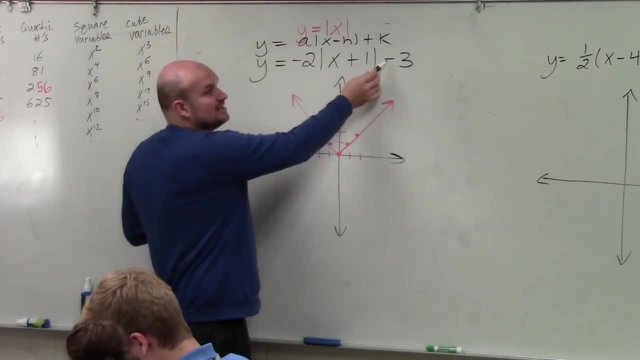 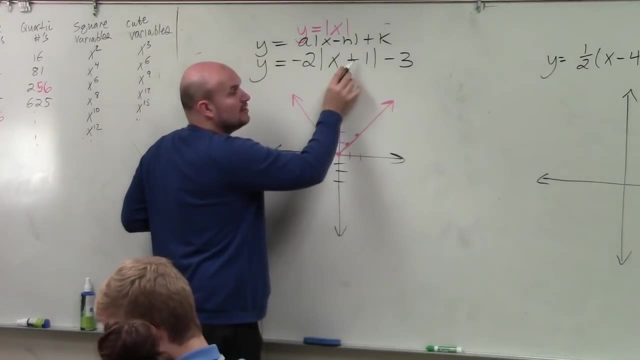 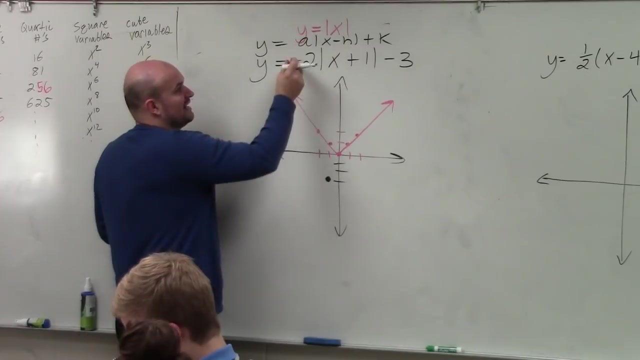 еня, the lowest point here on this graph, That was the point HK. So we can see the minus 3.. what is that doing to the graph? That is now shifting the graph down 3.. Then plus 1 is shifting the graph to the left one. And then the other important thing that I 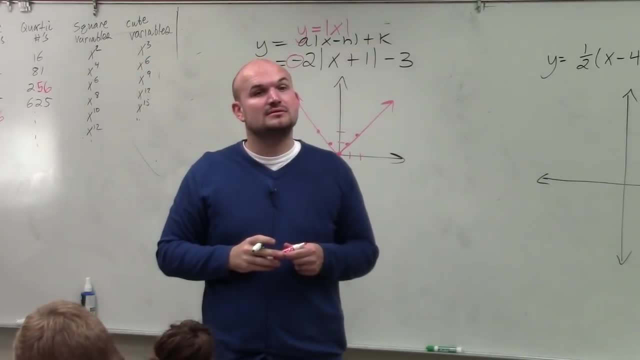 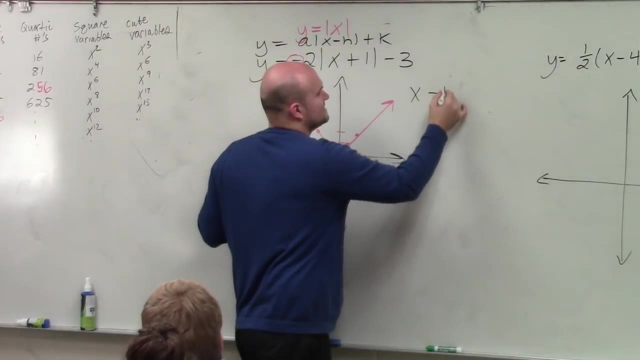 didn't say, but it's important is it's negative. yes, Yes, It's X minus H. X minus H minus. it's x minus h. x plus 1 is the same thing as x minus negative 1.. So what's the value of h? 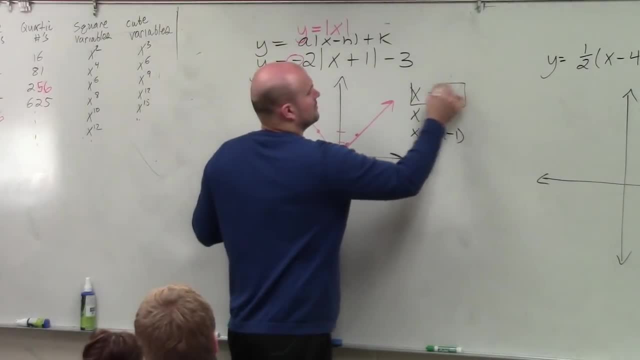 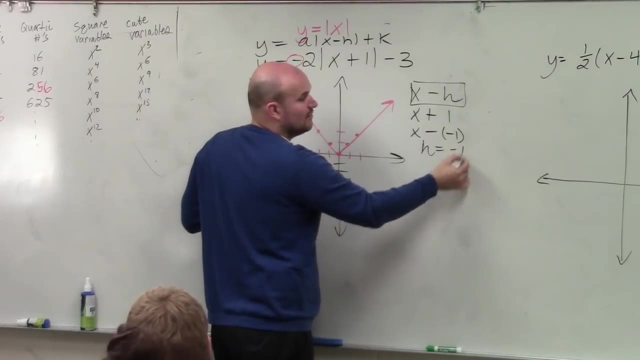 When it's x minus h, is the formula x minus negative 1. What's the value of h? h is equal to negative 1. So you go left. Just always think it's always the opposite inside the function. It's always the opposite. 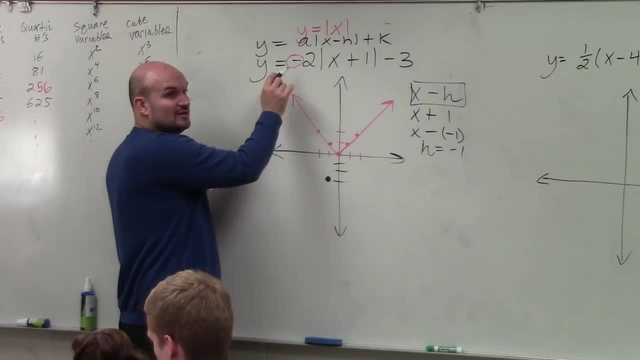 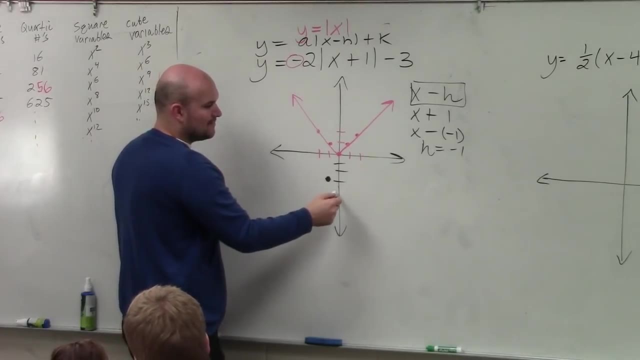 So that's why we're going to the left. This tells you to do what, though? Reflect down Instead of the graph opening up. the graph opens down Right Now. the typical formula for this was always: over 1, up 1.. 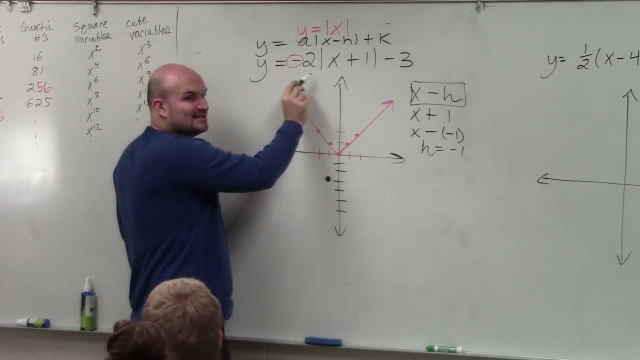 Over 1, up 1. Right, But now you're multiplying by 2. That is compressing the graph horizontally. So what we did was we could kind of thought about this as kind of like your slope in a way, This one. you can kind of think of it like that. 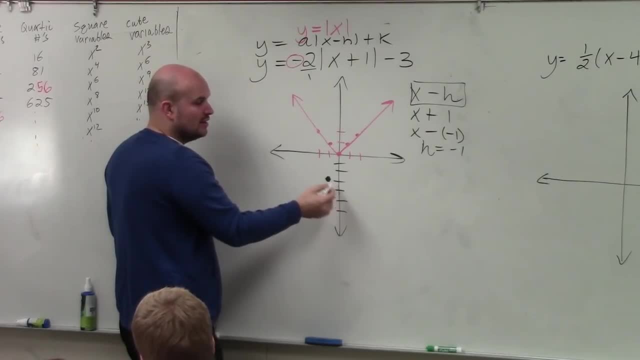 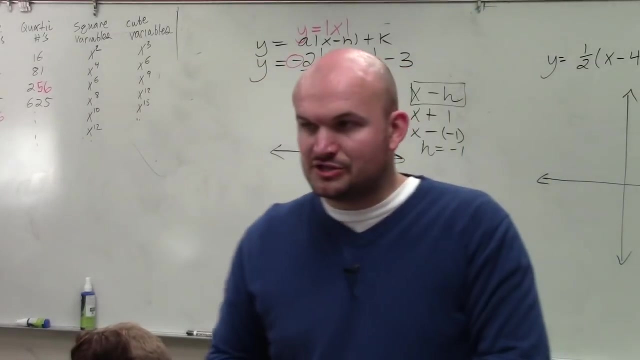 So now we go over 1.. Instead of going down 1,, we're going to go over 1, down 2.. Over 1,, down 2.. So the graph should look like that. Okay, I applied my vertical translation. 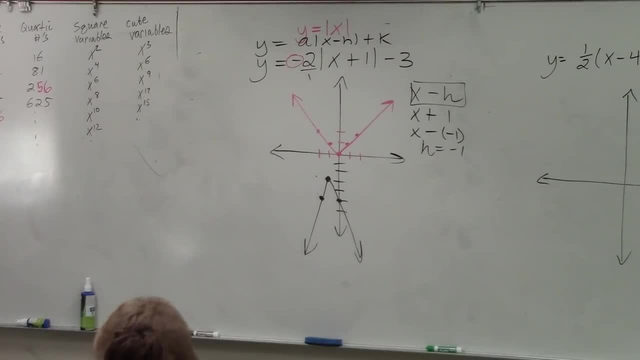 I applied my horizontal translation, I compressed the graph horizontally And then I replied the reflection.